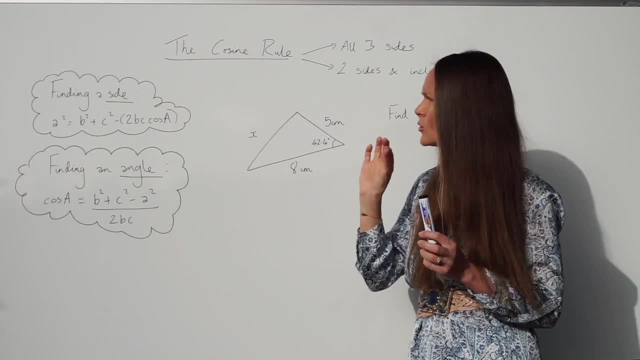 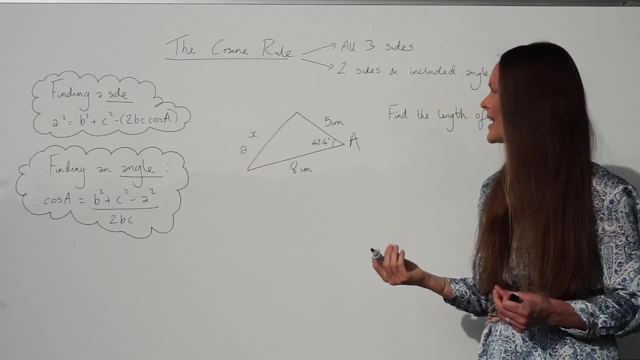 A. this would be the side little a. So those ones are important, So I'm going to label those first. So there's the angle, capital A and the side which is opposite, little a. Now when you label the other two sides, B and C, it doesn't matter which way round. 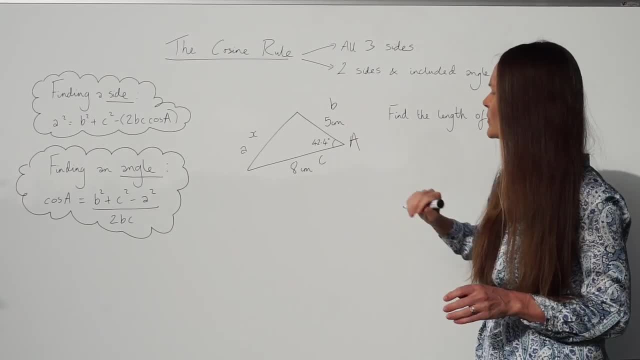 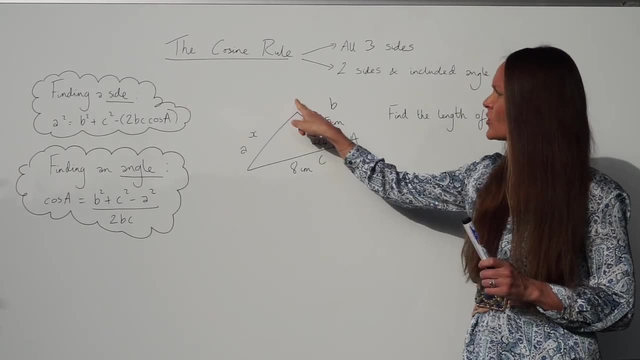 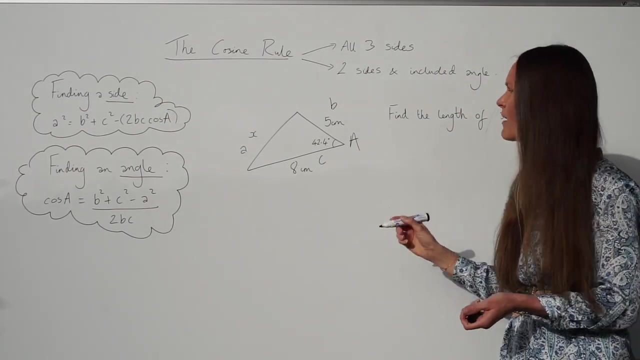 you label them. So I'm going to label this one B and this one C, And now it's really easy, You just substitute into the formula. So, because we're finding a side, I'm going to use this version of the formula. OK, so I'm going to start just by writing it down. 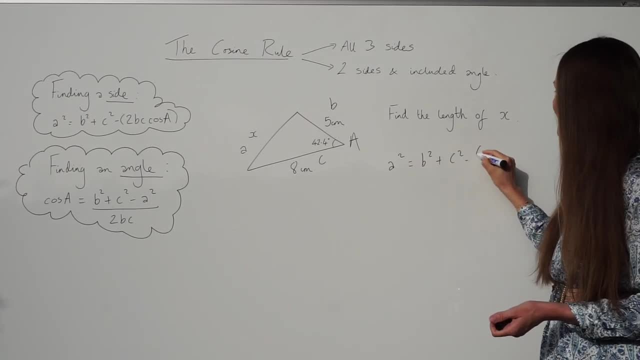 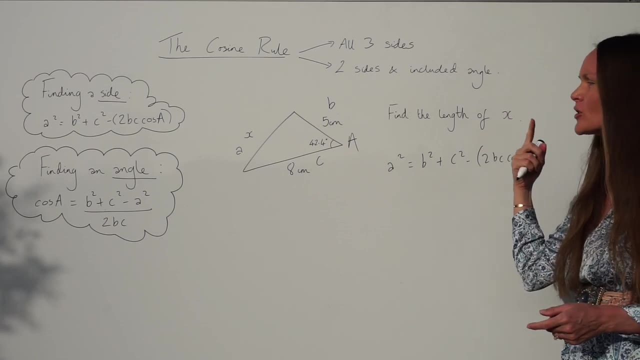 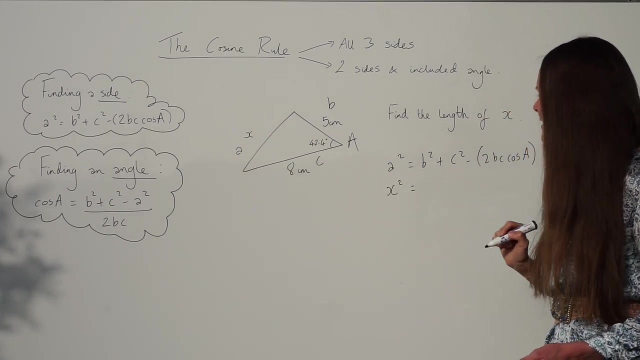 So A squared equals B squared plus C squared minus 2 times B, times C, times cos A. So I'm going to write it down And now I just need to substitute in the information given from the triangle: So little a is the same as x, So I can change that to x squared instead. 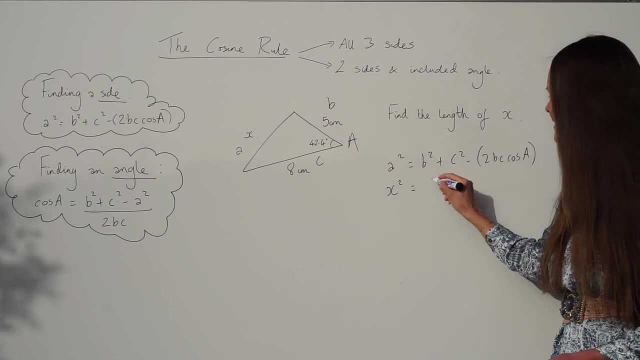 Instead of writing B squared, I can replace that with 5 squared. Instead of C squared, we can replace it with 8 squared, And then we have 2 times B times C, So 2 times 5 times 8.. Multiply. 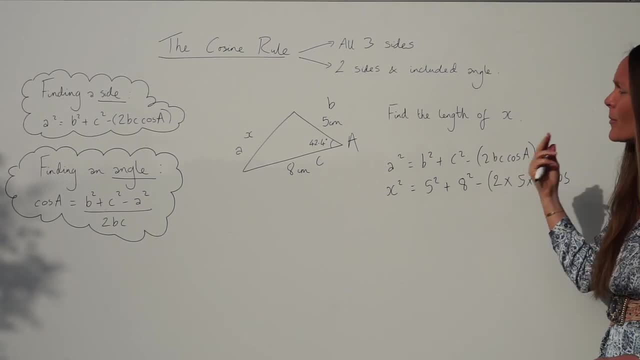 Multiply, Multiply by cos A And remember capital A is here. It's the angle. OK, 42.4.. OK, next, what I need to do is get rid of this squared on the x. OK, I want to find the length of. 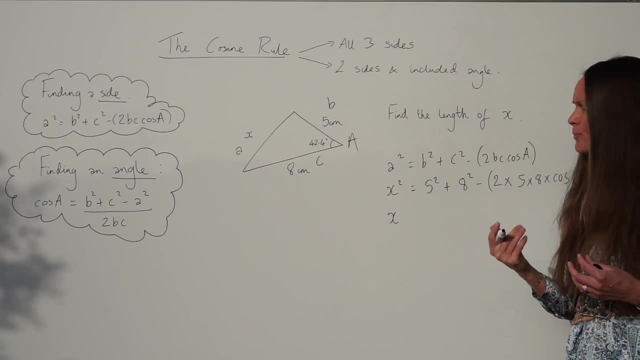 x. So to do that, I just need to square root both sides of the equation. So when I square root the left-hand side, it gives me x, which is what I need, And then I need to square root everything I wrote down previously. OK, so you're just putting this into the calculator. 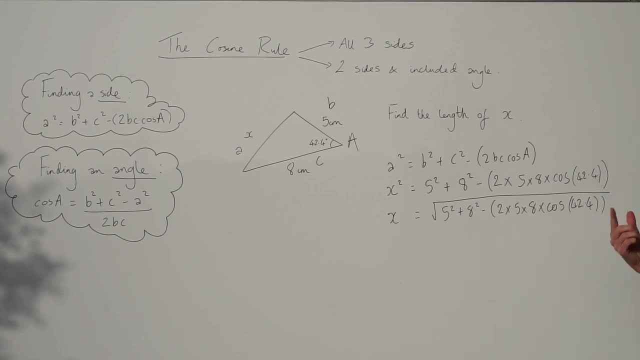 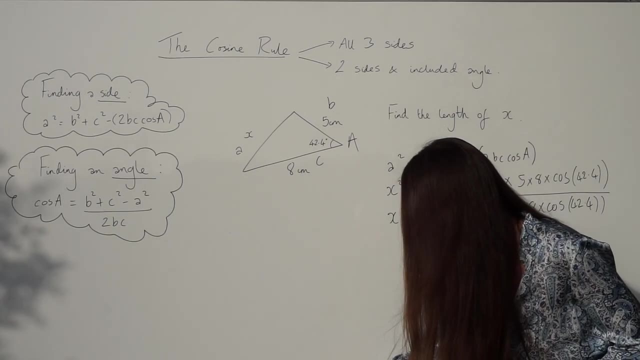 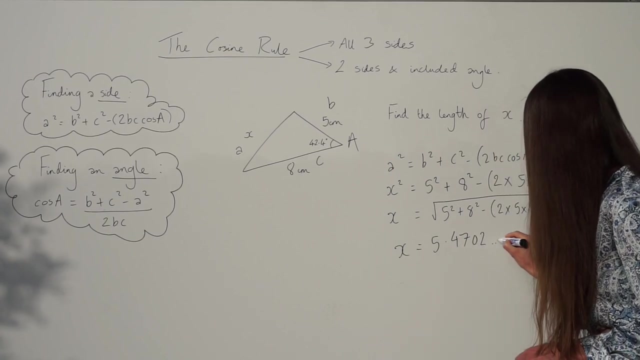 Just be really careful, when you do put that in the calculator, that you close your brackets OK, Otherwise you'll get an error on the calculator. So when you put that into the calculator, you should get 5.4702 and so on. Now just 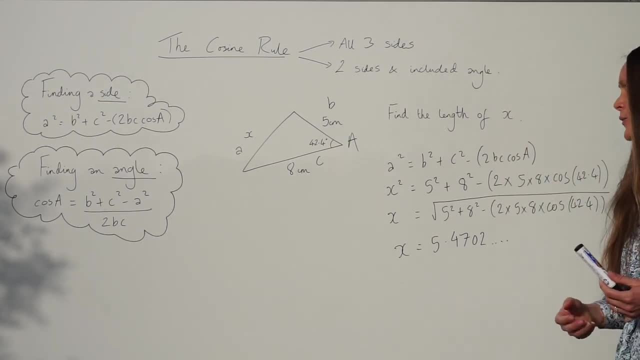 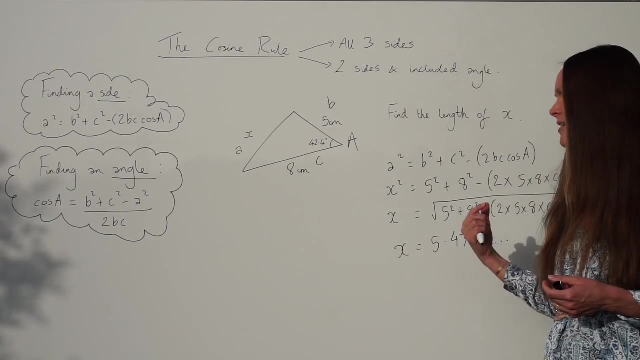 read the exam question carefully. You should get 5.4702 and so on. Now just read the exam question carefully that you've been given to find out how you're expected to round your answers. Usually, with the exam board that I use with my students, we round answers like: 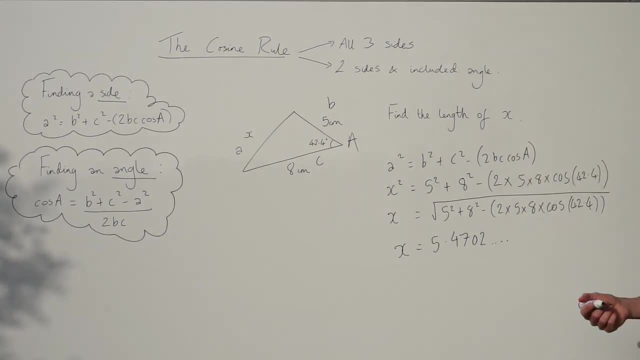 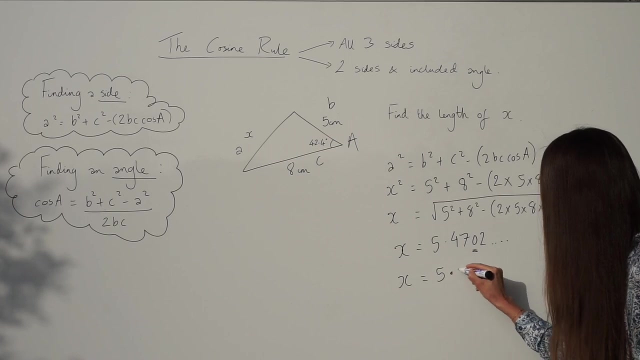 this to three significant figures. So I want three numbers in my answer: One, two, three. If I check the fourth one, because this is smaller than 5, it doesn't round this digit up. OK, It stays the same. So the final answer: the length of x is 5.4702.. 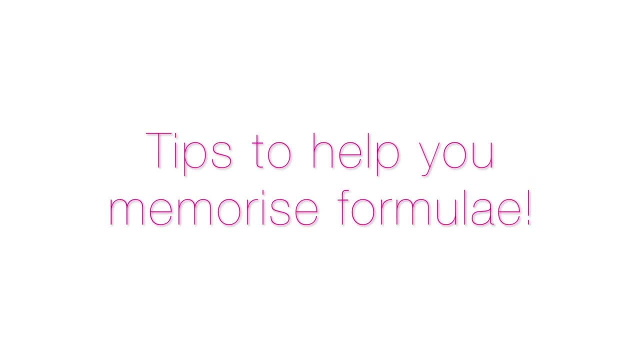 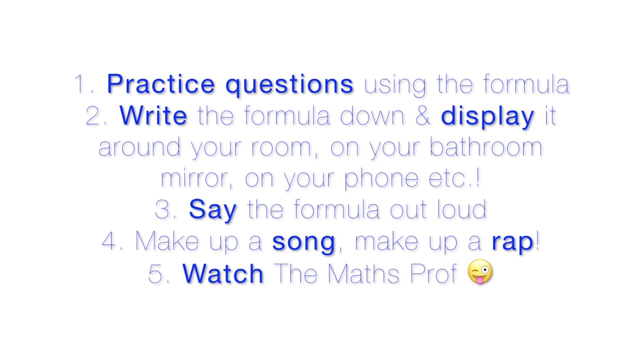 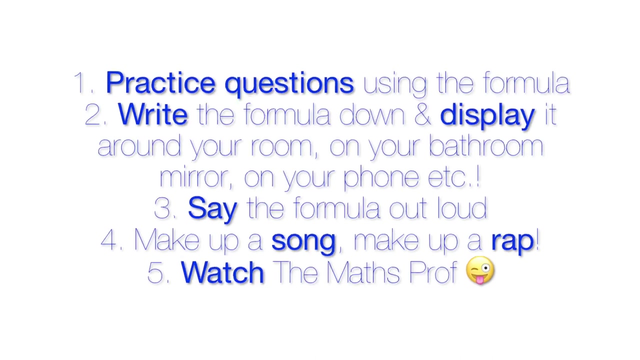 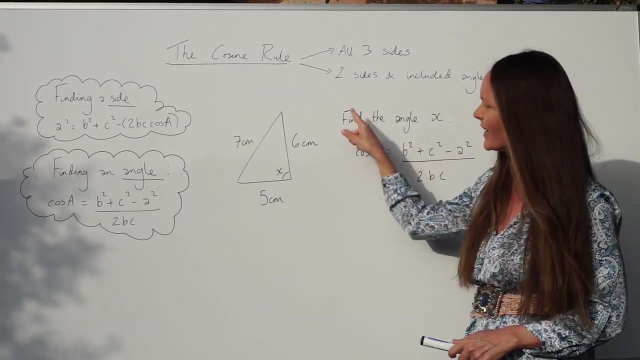 So the final answer is 5.4702.. So that's it for this. Let's do the next one. OK, so here I have the same answer. OK, so I'm going to go back and review this next question. OK, so I'm going to go back and review this next question. 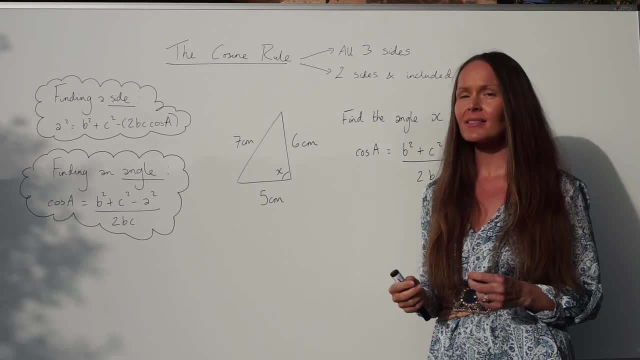 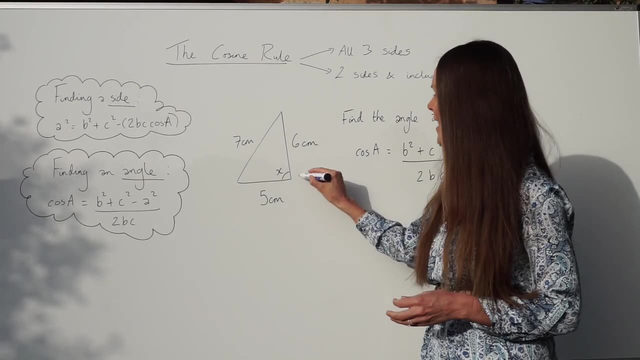 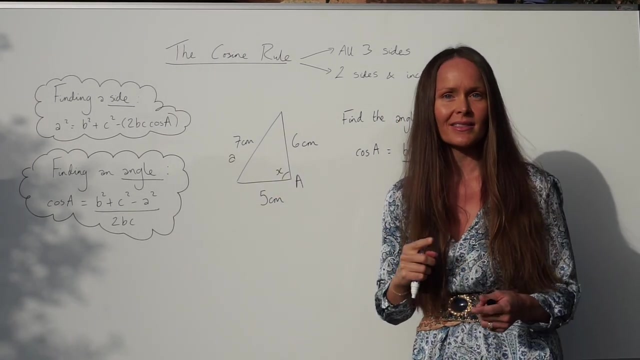 sides of this triangle. So, just like before, start by labelling your triangle. OK, so label the sides and label the angle. Remember the angle we label as capital A, which means the side opposite here is little a. And then, when we label the sides B and C, it doesn't matter. 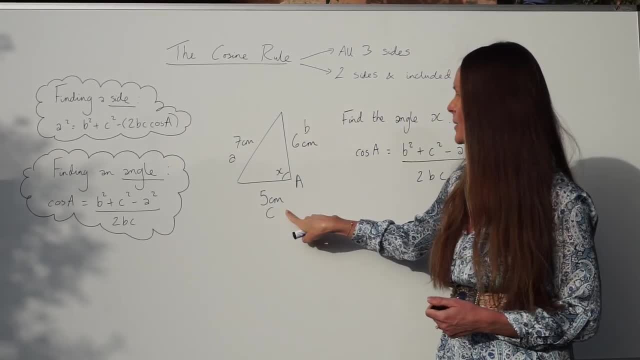 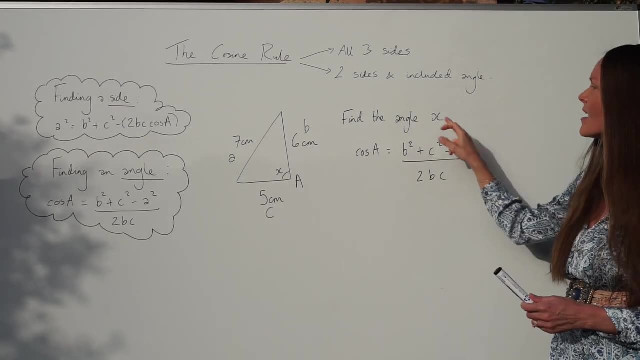 which way round you label those. I'm going to label this one B and this one C. So, because we're finding an angle, we need to use this version of the formula OK, which I've written down here, And then you're just substituting in the information from here into the formula. 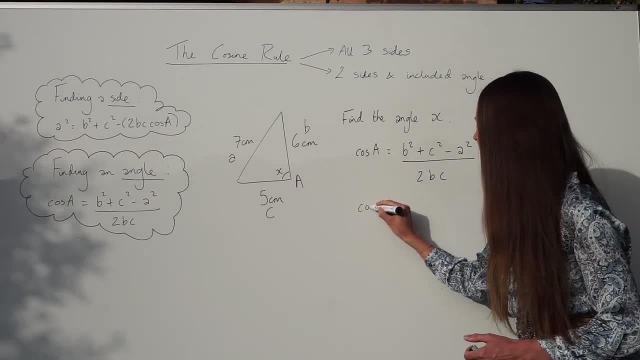 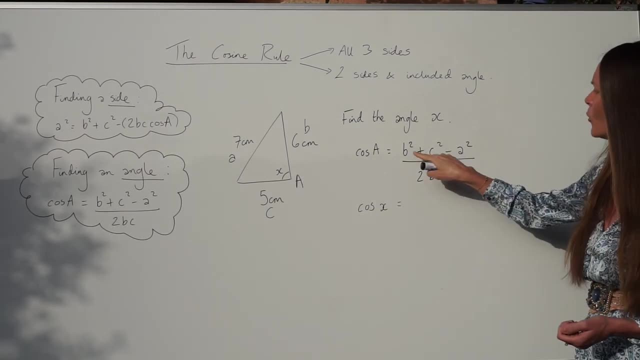 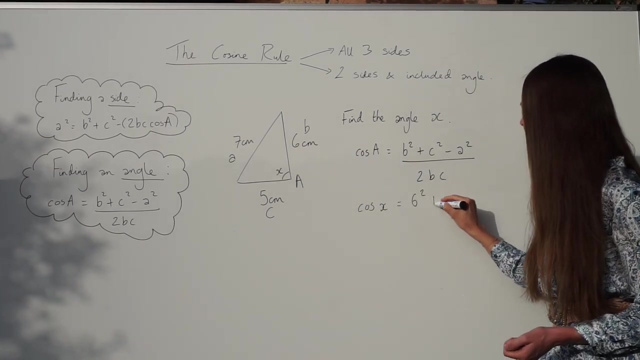 OK. So instead of writing cos capital A, you could write cos x. OK, because this is angle x, But it doesn't matter if you leave it as a. But all of these we're going to change. So instead of little b squared, I'm going to write 6 squared, Instead of C squared. 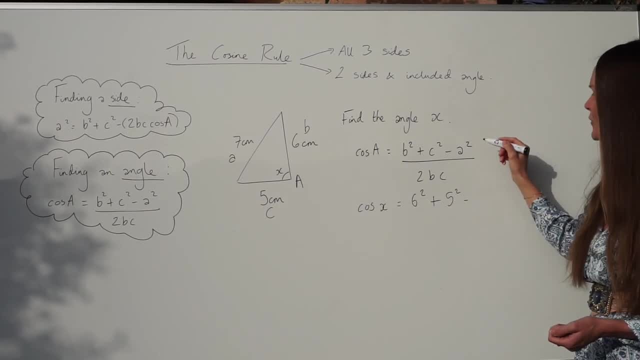 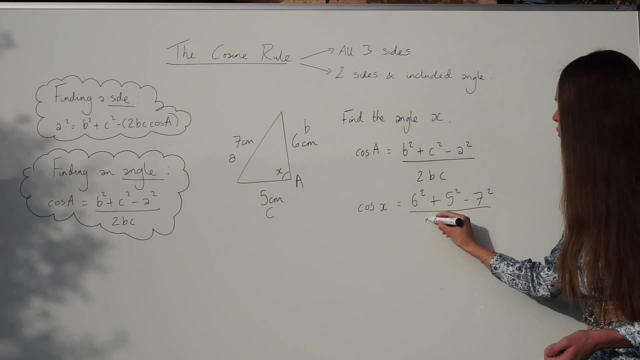 we now have 5 squared, And then we have to minus a squared, So minus 7 squared, And all of that is divided by 2, multiplied by B, multiplied by C, So 2 multiplied by 6, multiplied by 5.. OK, so you're literally just substituting in the 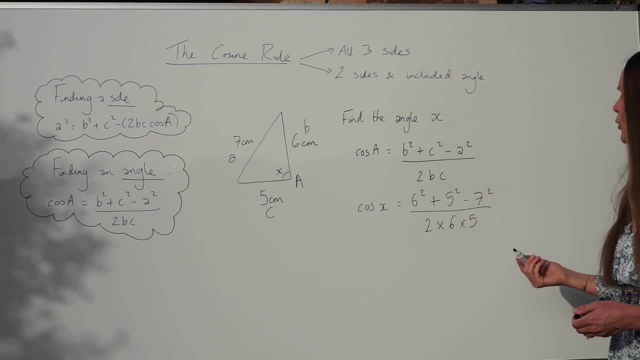 numbers into the formula. OK, Now when you put that into the calculator, you get 0.2, OK, So that can't be the angle. OK, That's a strange answer for the angle in this triangle. If we look back here we can see that the angle in this triangle is 0.2.. So if we look